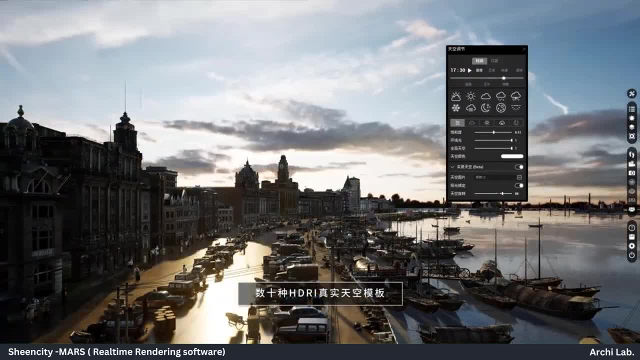 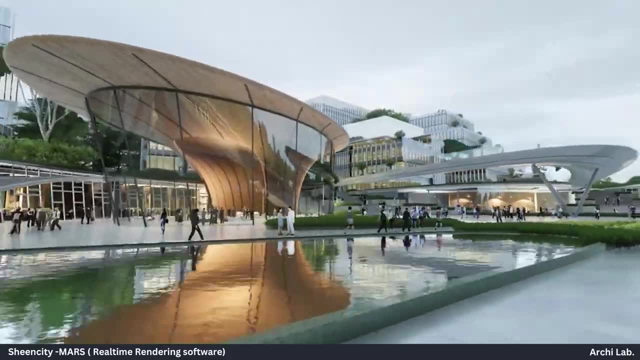 including functionality. If you are interested in this software, visit their official website.